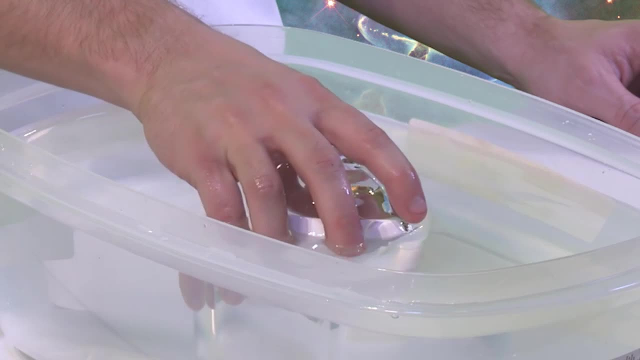 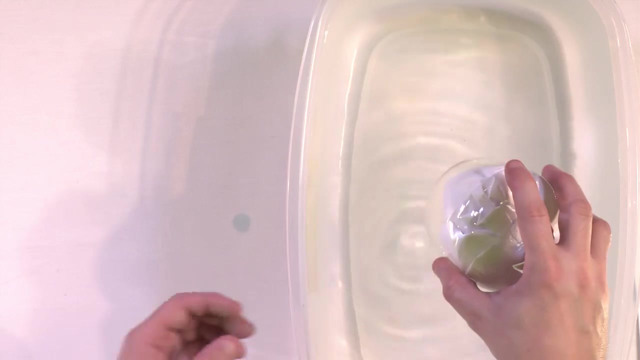 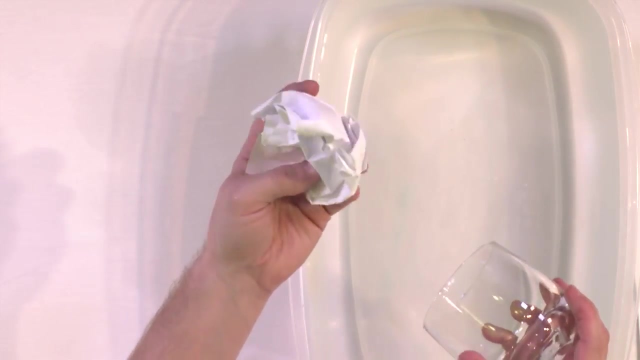 four, five, And then you gently lift it up And then you go tap any excess water off of there, And then you gently reach in and pull your paper out, which is completely and totally dry. It is not wet at all, And so you've won. 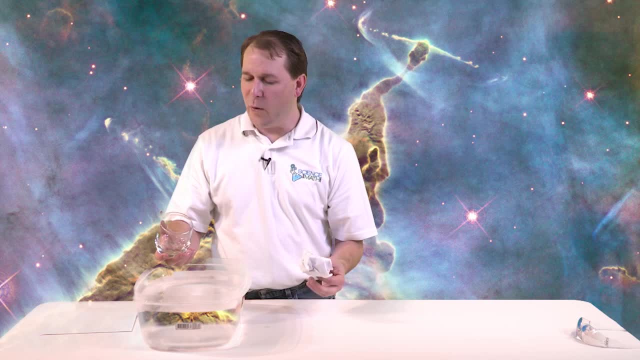 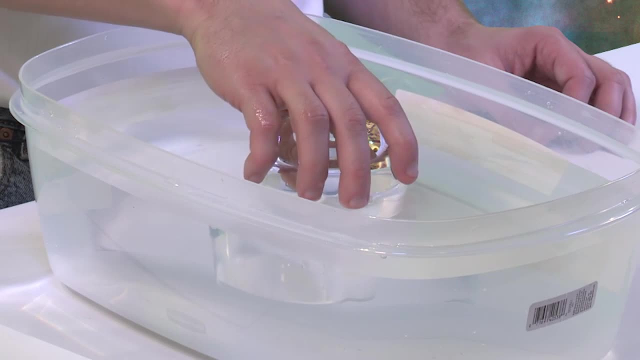 the bet right, So you go ahead and get paid up for that. Now, the way this works is really interesting. So what you have when you put any kind of cup upside down under water: it kind of looks like it's filling up with water, but it's really not filling up with water. 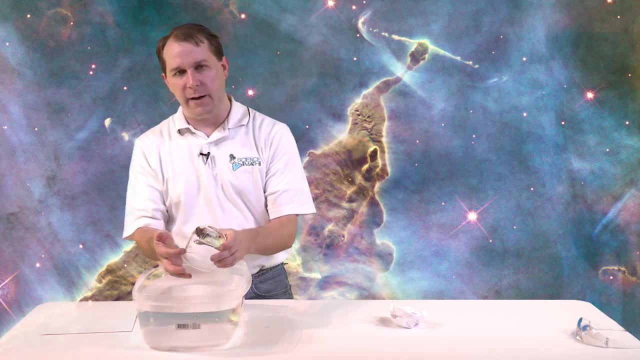 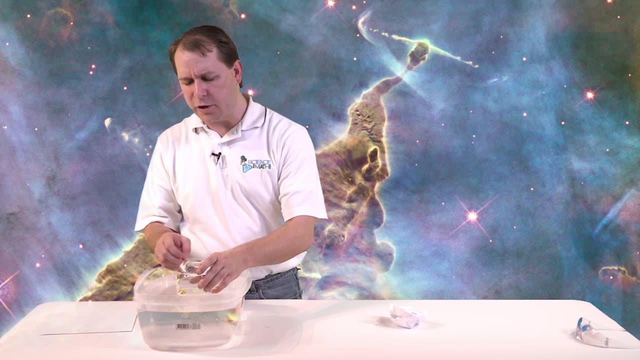 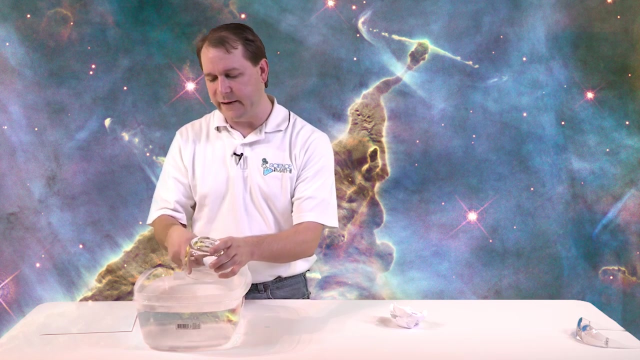 It is full of air. So there's air inside this cup. right, There's air all inside this cup And whenever you put it on top of the water, there's air pressure inside of this cup here because there's air in there. That just means the air is pushing against the walls, pushing against the inside. 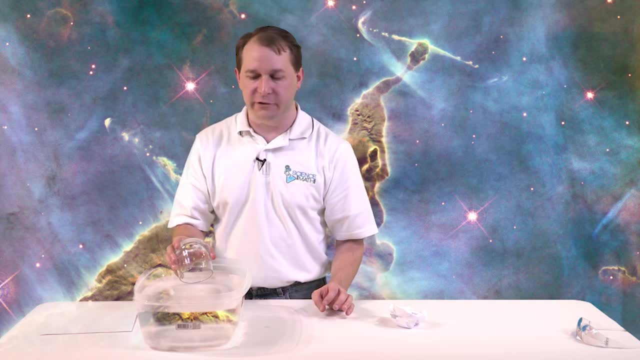 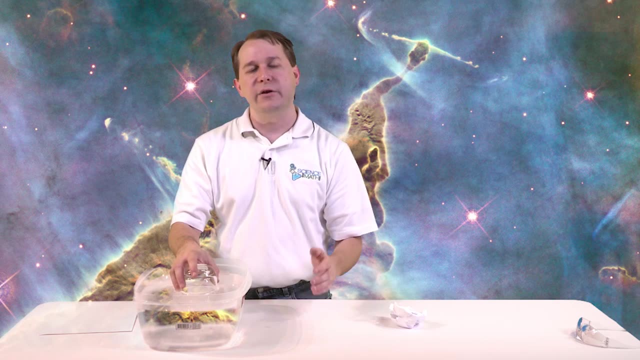 pushing out Anytime you have air in there, you have air pressure right. So that's trying to make the air come out, but there's this water underneath it and that water is trying to come in, And so you have a balance of the forces. 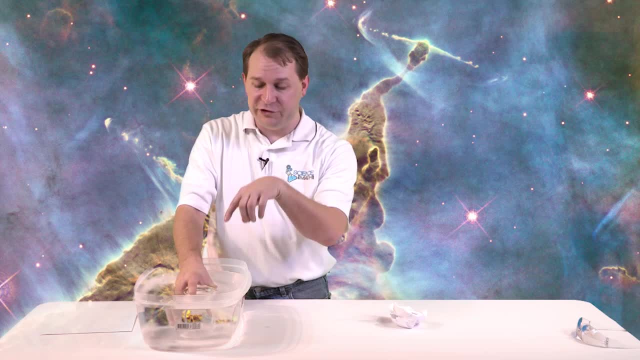 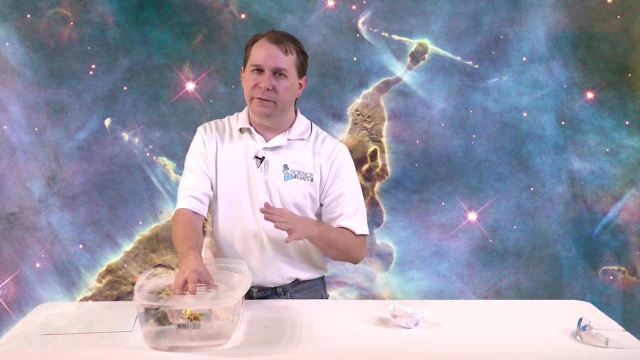 You've got the inside air pressure trying to push the air out, So it's trying to expand and push the air out, but you have the water pressure underneath, The water is trying to come in, And those two things are more or less balanced right now, And so that means 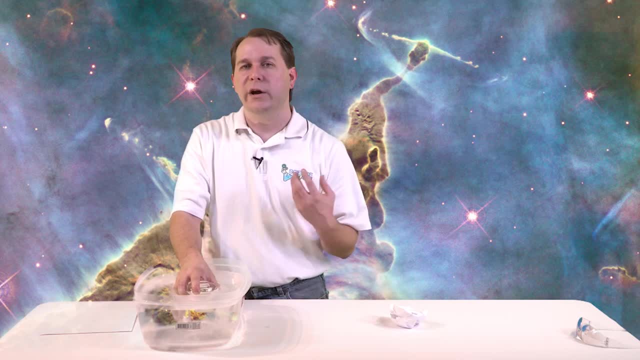 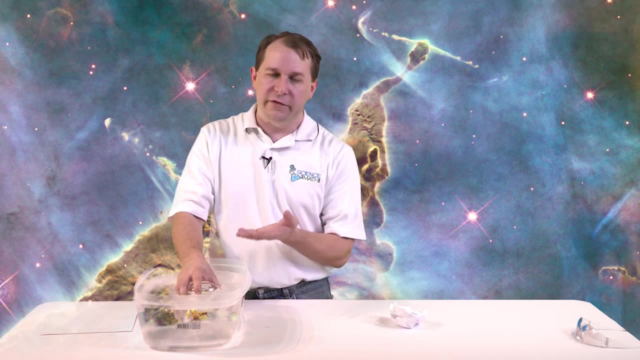 that the air is going to stay on the inside, the water is going to stay on the outside. We always think that the water is going to force its way in, but it can't just force its way in. It has to be able to overcome the air pressure. 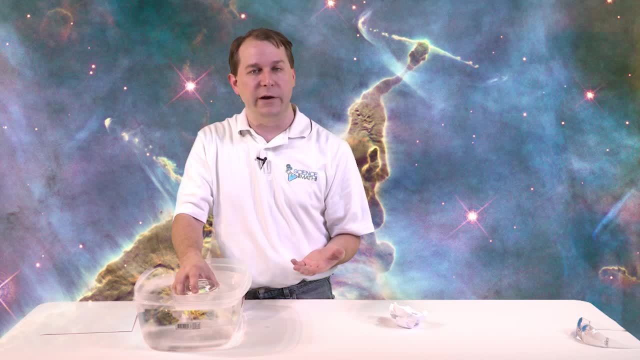 So again, it's a good example of why you can look at a real life situation and understand that air really does have a balance. So you can see that the air is going to stay on the inside. It can't just push the water out. So we're going to look at a real life situation. 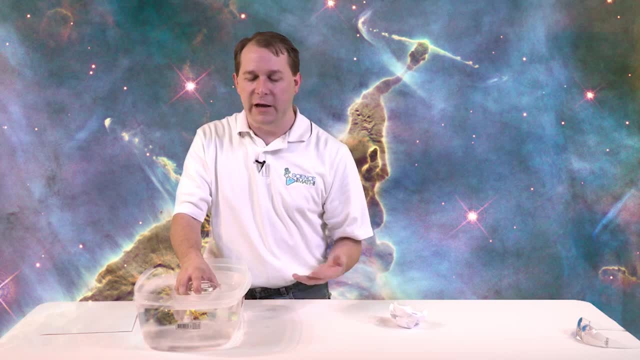 now. So we're going to look at a real life situation now, So you can see that the water is going to push the air out, And that's a good example of why you can look at a real life situation and understand that the air is going to push the water out. 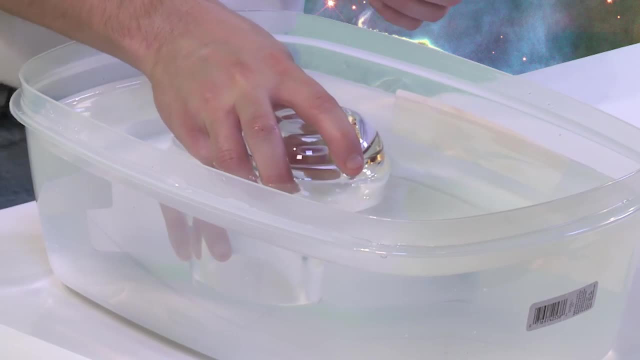 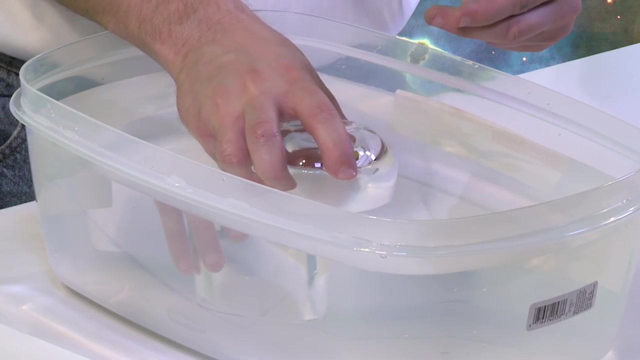 So if I go under water and I gently tilt this cup, Now look what happens whenever I gently tilt this cup. When I tilt it, some of the air can actually come out and bubble up the side and then some of the water can rush in. So if I go under water and I gently 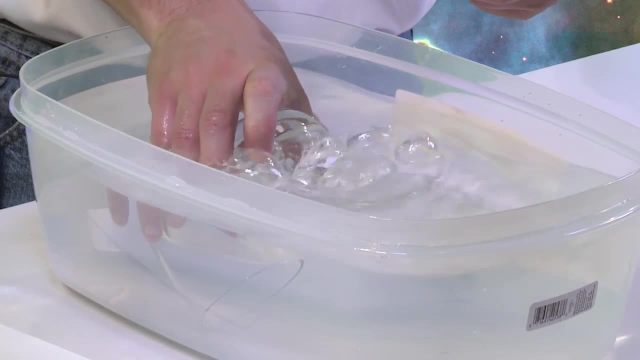 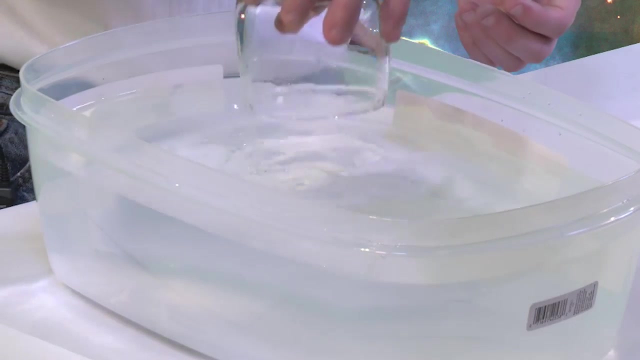 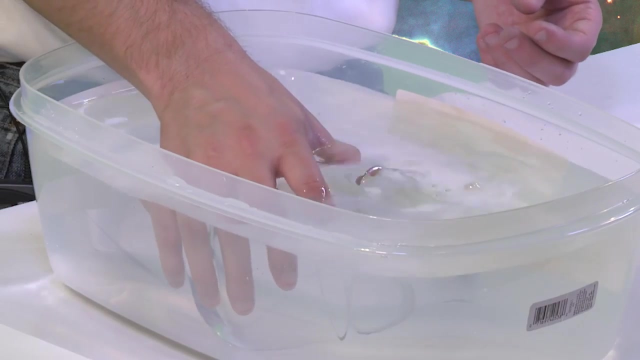 tilt it, then I get lots of bubbling And then, of course, I have the water going into the cup. Now another thing you can do: you can go under water with it. you can let water in like we do, and I think most everybody here has probably done this in the 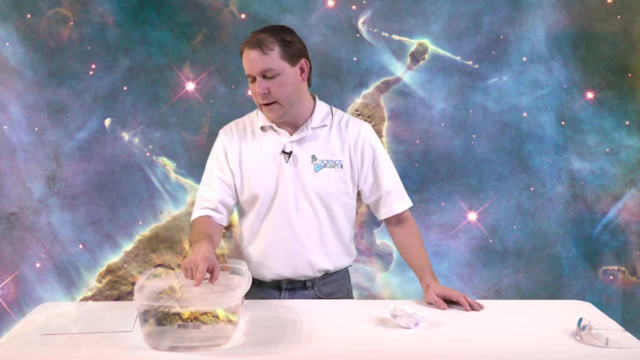 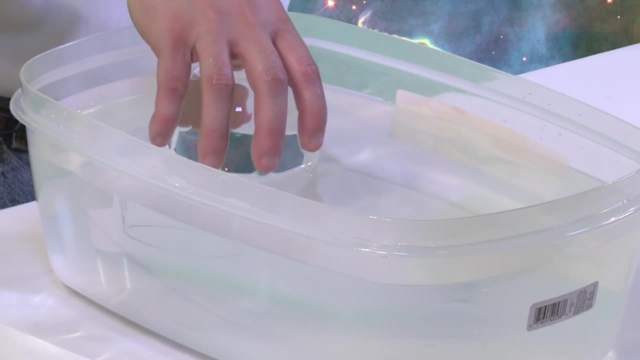 bathtub at one point. so now we have the glass of water underwater and it's completely filled with water, right? so there's no air in there at all anymore. now, whenever we lift it up right just above the water line, then what we're- what we have here now- is the glass is full of water, but the 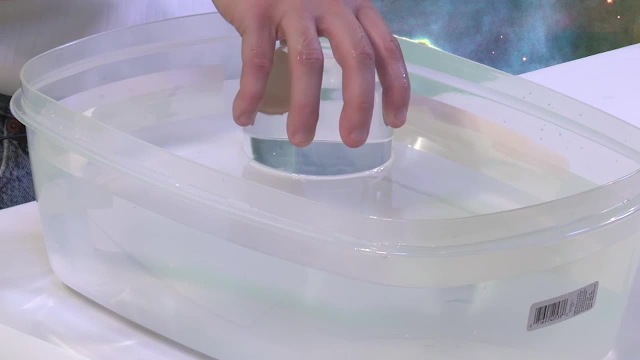 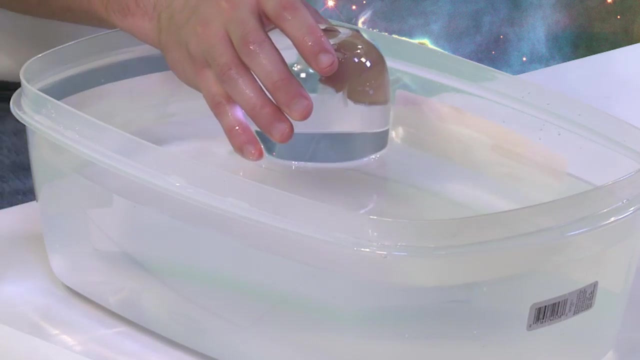 glass of water. the water is not, it's not leaking out and it's not going back into the container of water. why is that? it's exactly the same thing. it's, it's pressure, so there's, there's water inside of here, and that water has weight and it's trying to push its way out through the bottom, but there's. 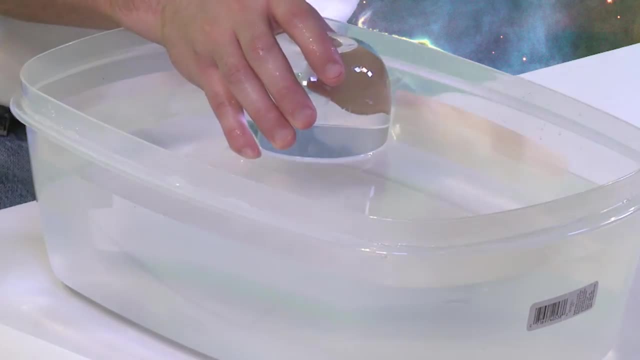 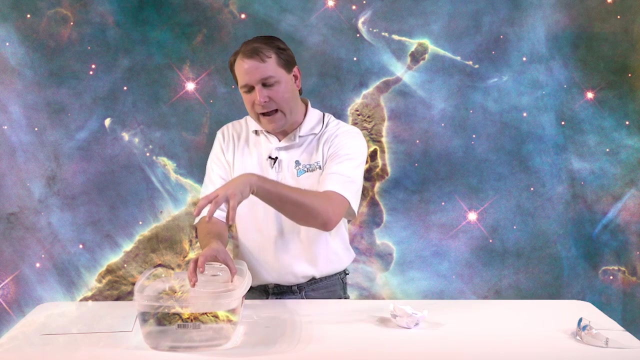 air pressure all around this entire vessel of water. the air pressure is pushing on top of this water and trying to push its way back into the cup. so you have an inside force- the gravity- pulling the water down, and you have an outside force which is pushing on the top of this water here. 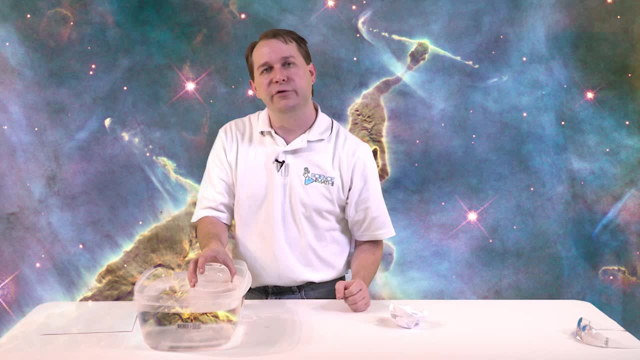 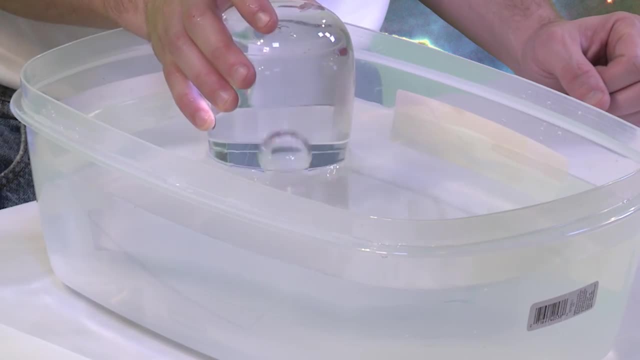 trying to force it, basically force it back up inside, and those two are in balance and so everything is in in check until you just lift it barely out of the water to let some of that air in and some of that water to go out, because as soon as you lift it outside the 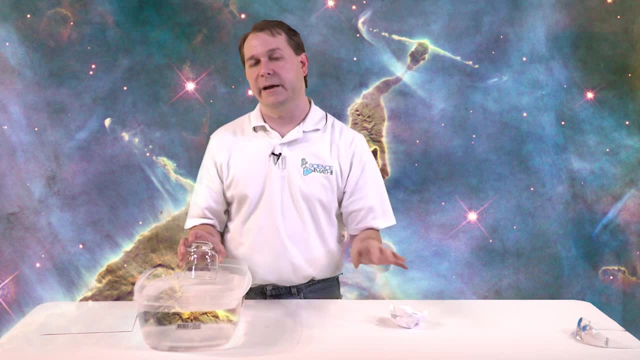 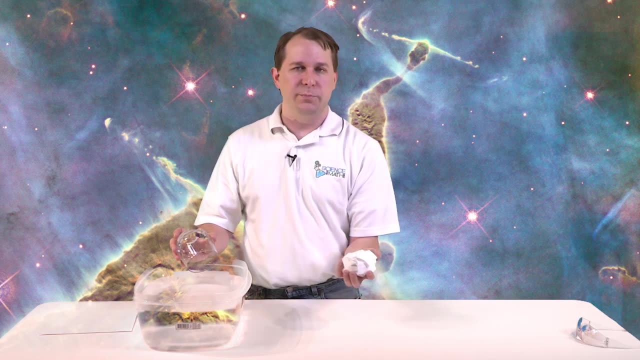 water, then basically the air is allowed to come in, that that pressure is allowed to become, though there's no pressure anymore because there's no water anymore. so it's kind of two experiments in one. first you put it dry glass, dry piece of paper in there and you didn't say exactly. 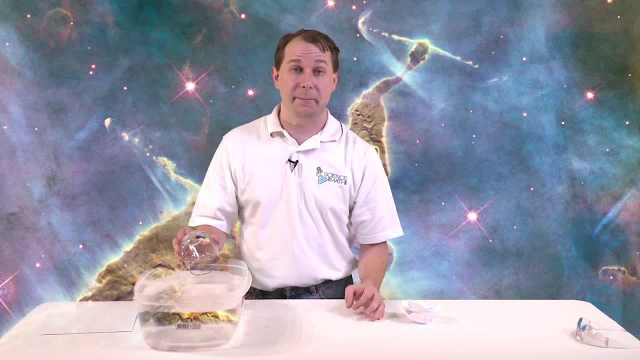 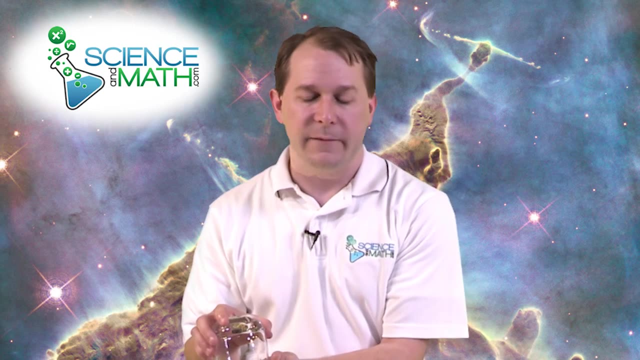 how you would do it. you just bet somebody that you could put a piece of paper in there and you put it under water and it would stay dry. that's exactly what you did: you put it under water and it stayed dry. you created a pocket of air where there was pressure inside that kept the water out, right. 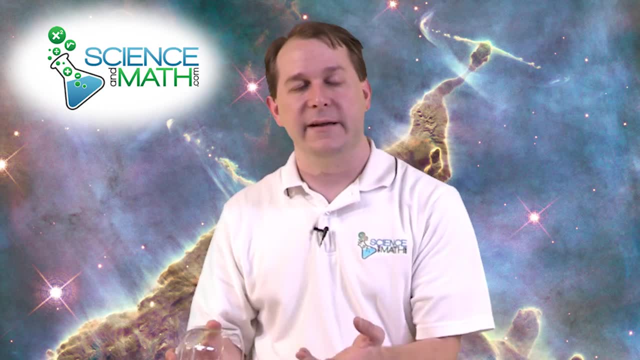 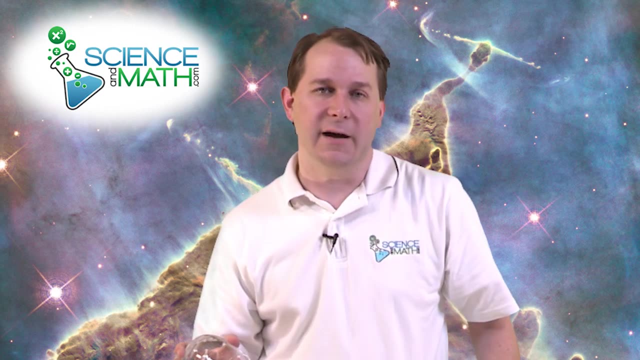 and then the other thing we did was we filled it up with water and raised it up and sort of a similar thing happening: the outside air pressure is pushing on the on the water on the outside, keeping that water inside of this cup whenever you lift it up. so very simple stuff to do, but you know, always take. 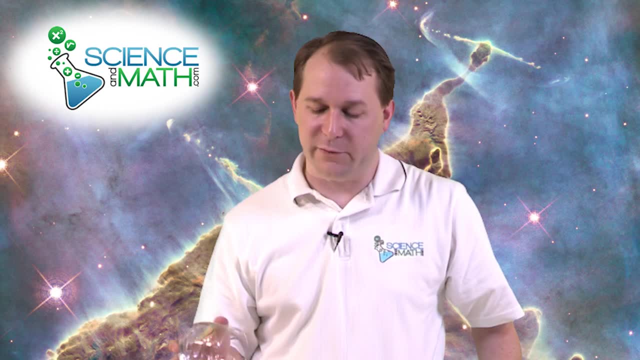 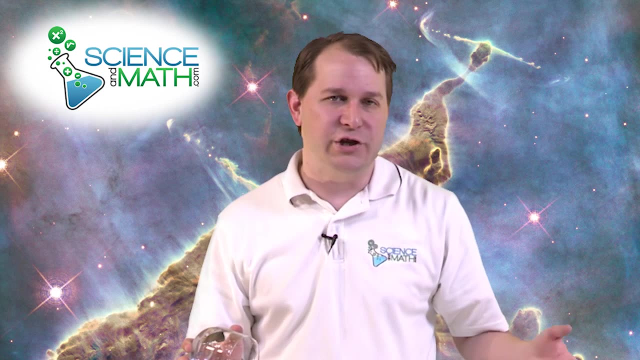 time to make sure you understand what's actually happening, and that's what we did today. so go grab, grab these materials, have fun with them and have fun showing people that you know a little bit about air pressure and how you can use it to take a piece of paper, put it. under water and have it stay dry.